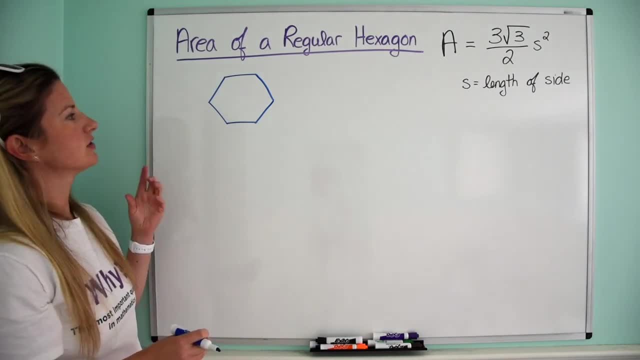 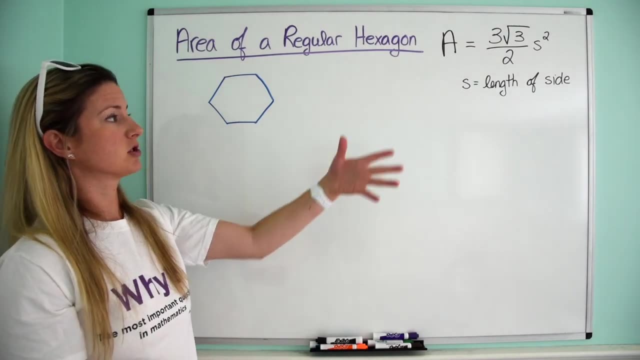 bad. So the area of a regular hexagon. so it has 6 sides. Because it's regular, all those sides have the same measure. okay, So because we know our formula uses the length of the side squared, we're just going to call every side here s okay. 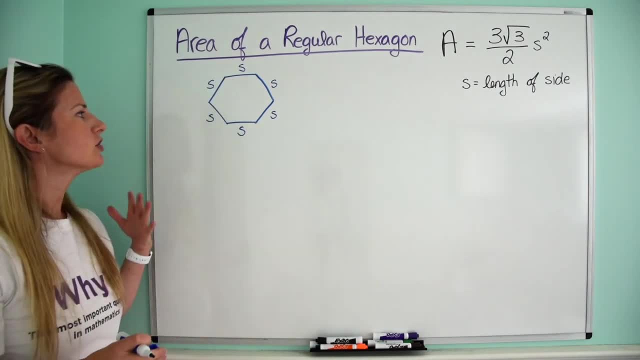 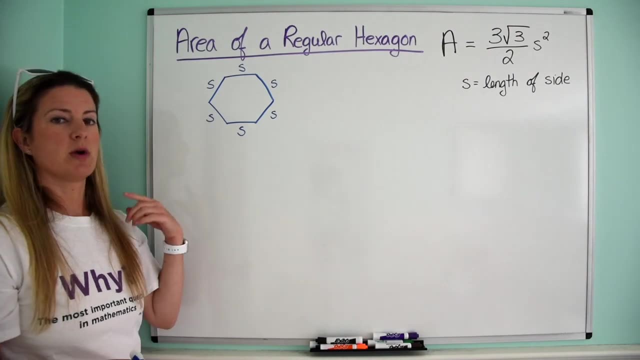 All right, so I want to try to figure out how to find the area of this, but instead of using- like in my video, where I use 7, we are going to use s okay, So the first thing I'm going to do, 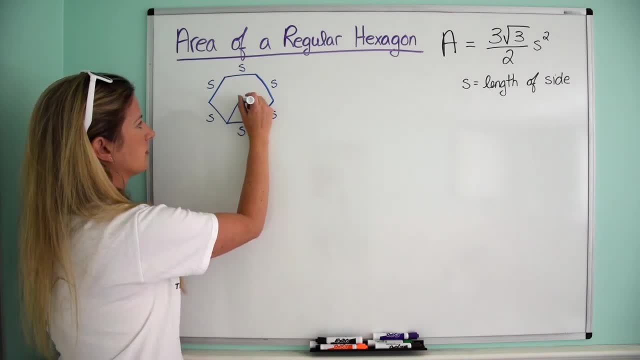 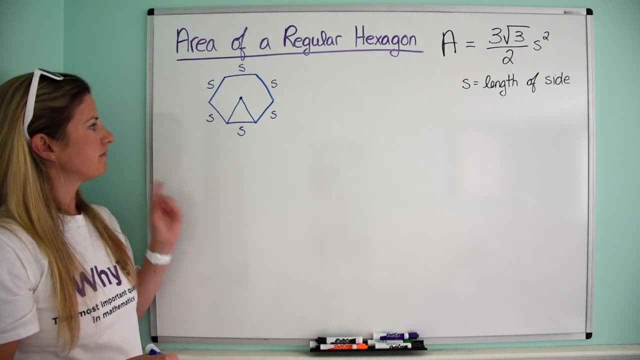 is going to put a center, a dot in the center, and talk about a triangle. Because what's so super duper important is that if we can find the area of the triangle, we can just multiply by 6 and get the area of the whole thing. So it's you know, it's going to be a lot easier to find the. 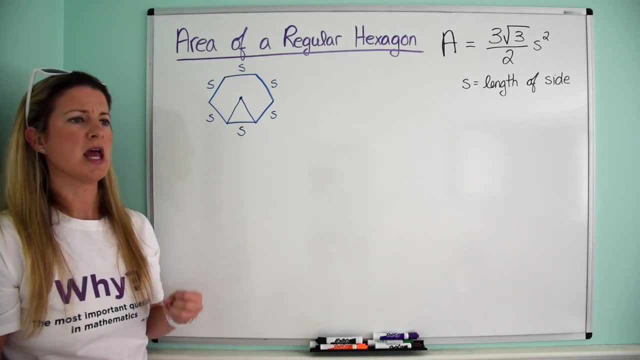 area of the triangle. So it's super important to think of, like, how we can break something up. okay, Triangles are your friends, especially 30,, 60,, 90, and 45,, 45,, 90,, because you don't need a. 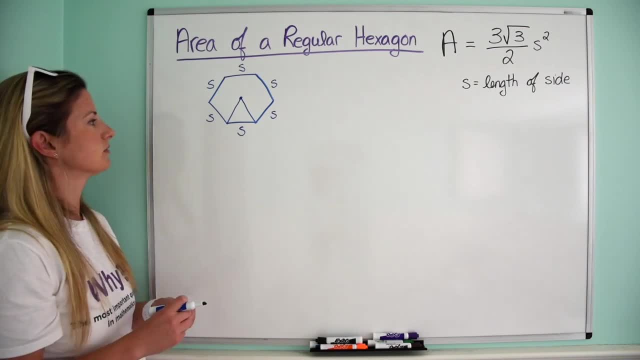 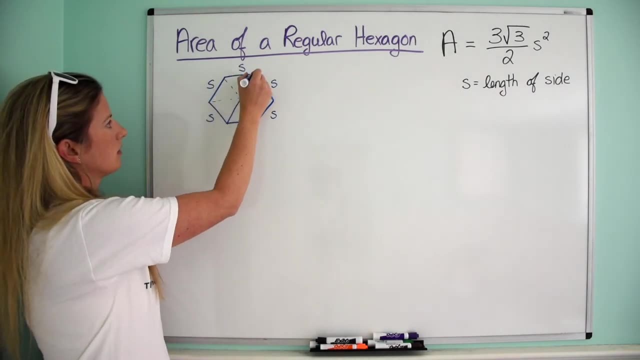 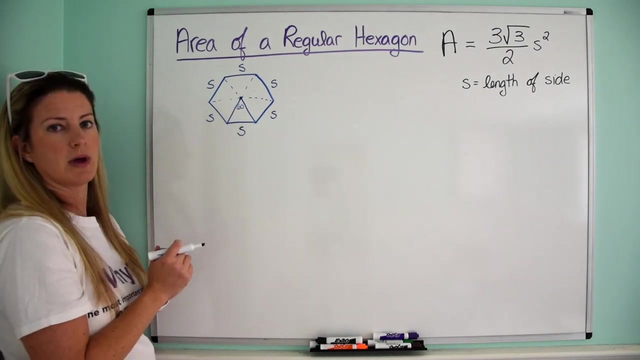 ton of data to be able to, you know, find the missing pieces right. You just need one side. So when I have a hexagon, remember if I were to draw out, okay, all these other segments here. I know I have 360 degrees, Because I have 6 of them. I know that this is 60 degrees, okay. 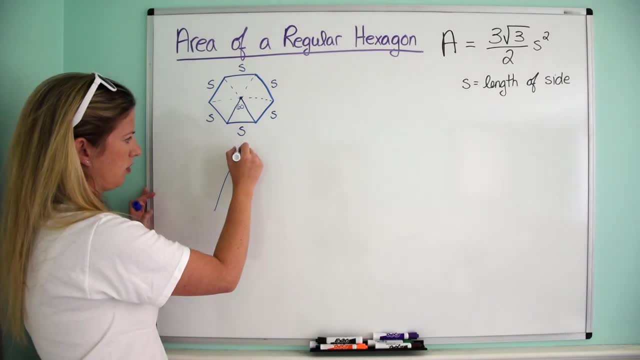 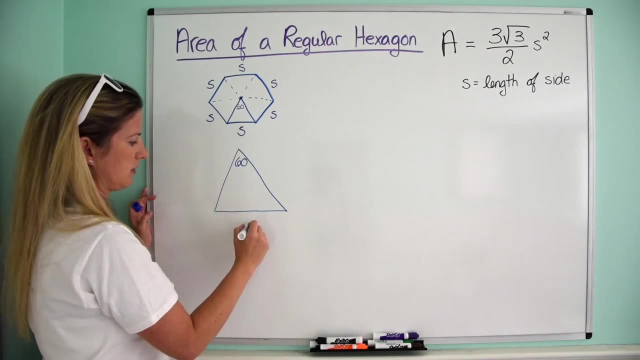 So, just to make things easier, I'm going to use a hexagon. So I'm going to use a hexagon. I'm going to pull this triangle out right here, okay? So I'm taking this triangle and I'm doing it right here, just so that we can see it better, okay? So, remember, this was S okay. Now I'm going. 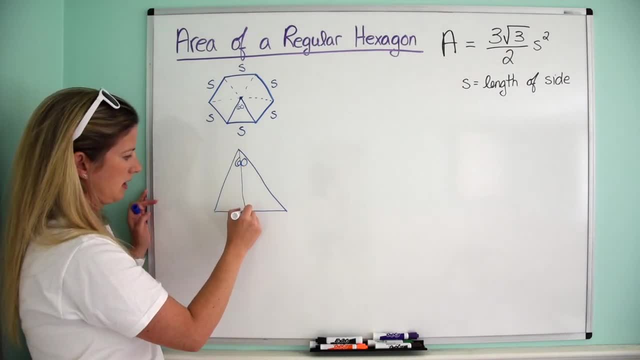 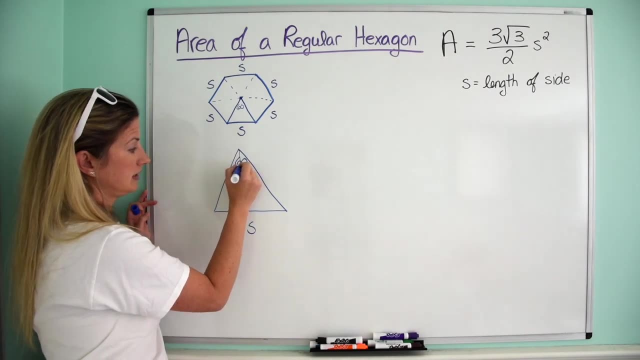 to drop an altitude, okay. So when I drop an altitude, it's going to bisect this angle right here. So, instead of this being 60,, this is going to be 30, and this is going to be 30,, okay So? 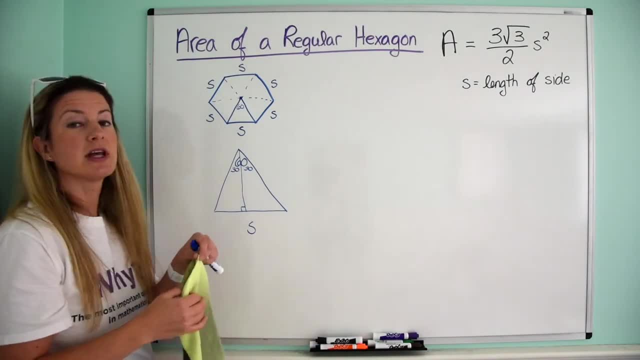 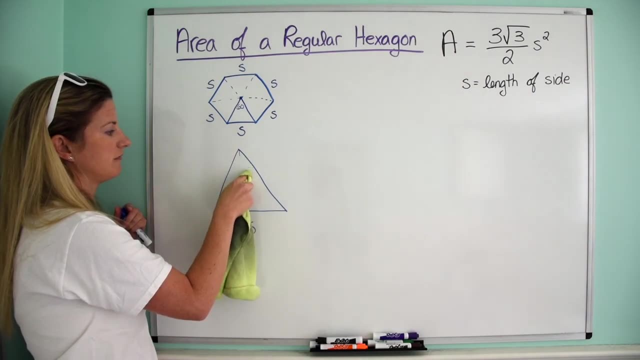 if I want to make it a little even more clean, because, remember, your teacher says: always do math in pencil. and you should, because sometimes you want to erase things to make things less busy, if you will, so you don't get confused. okay, Because we replace. 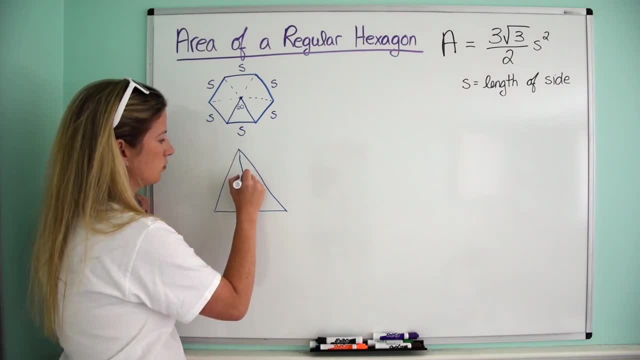 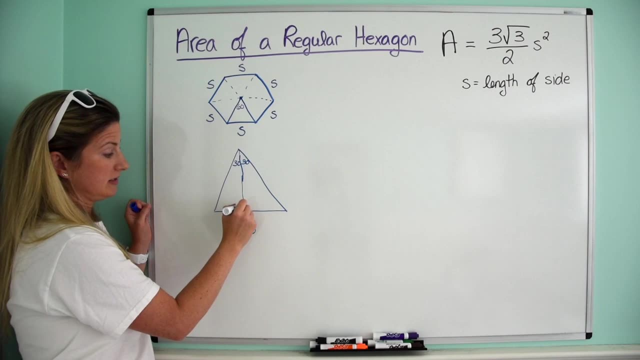 a lot of things, sometimes with other things, Okay. so remember, this was 60,. okay, And now I have bisected it when I dropped that altitude and I've got 30 and 30. Remember, this is 90,, so this is 90.. 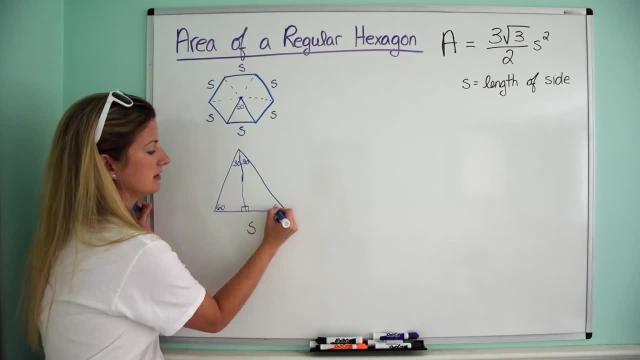 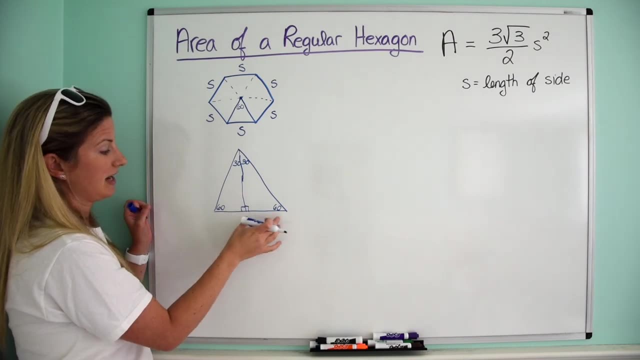 So that means this must be 60, and this must be 60,. okay, So I've created- because this is an equilateral triangle, And then I bisected that angle. This is also going to bisect this side. I know visually it doesn't. 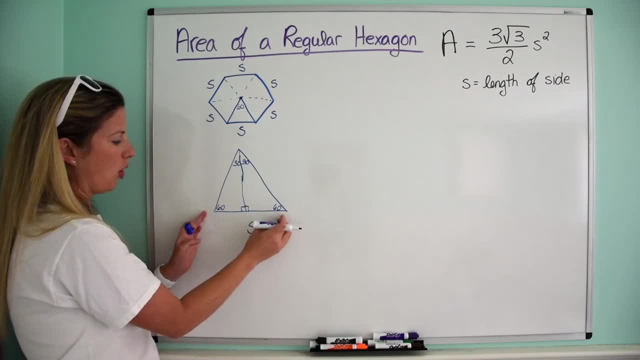 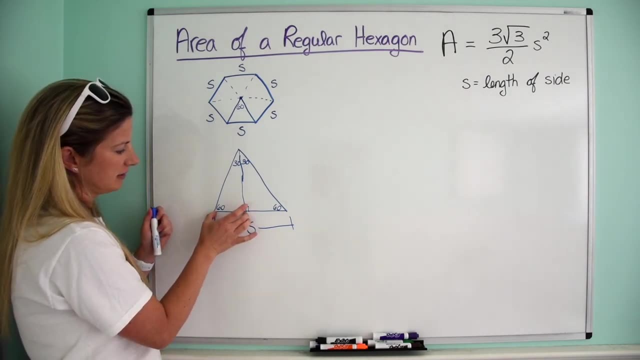 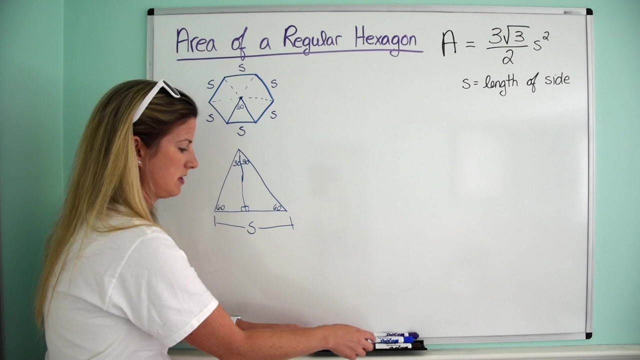 look like I bisected it, but that's what's going to be happening here. So the whole thing is S okay, But each little piece here okay is going to be what? One half S, So if I take maybe. 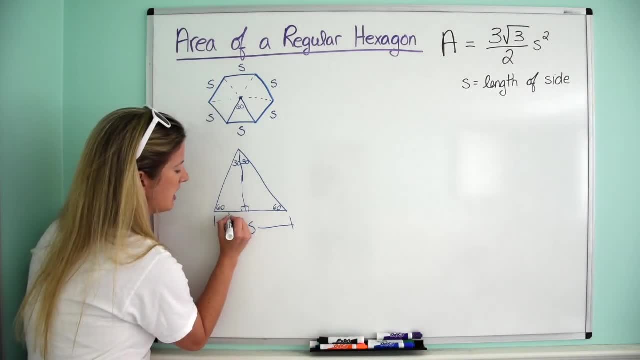 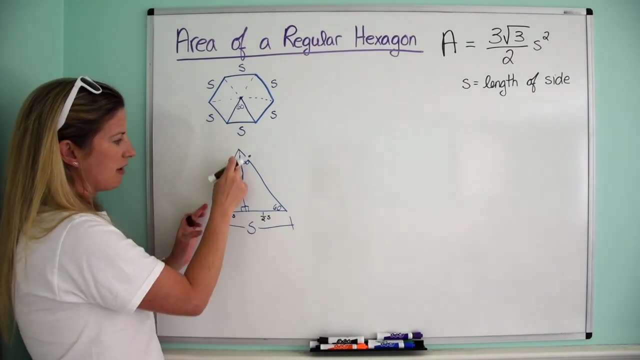 I don't know, maybe the I'm just trying to show it in a different color. So this is one half S and this is one half S. One half plus one half equals the whole thing. okay, Now, the reason I wanted that was because 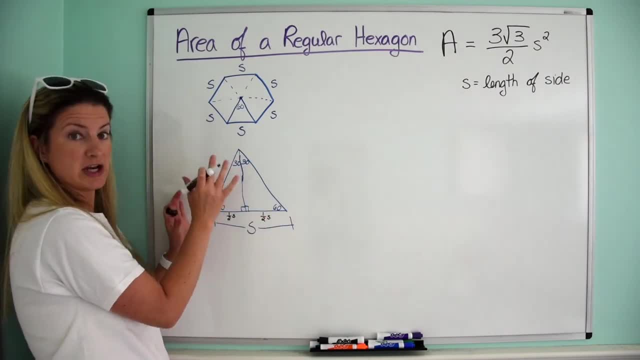 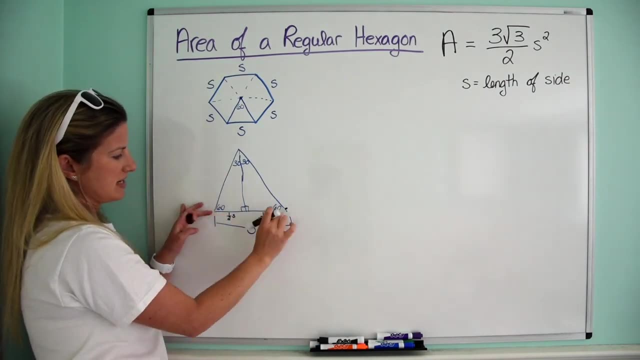 in order to get the area of this triangle- which, remember once, I know that I'm just multiplying by six to get the area of the whole hexagon. okay, To get the area of this triangle, I need the base, which I have, which is S, and I need the height. okay. Now you might be thinking: well, why did? 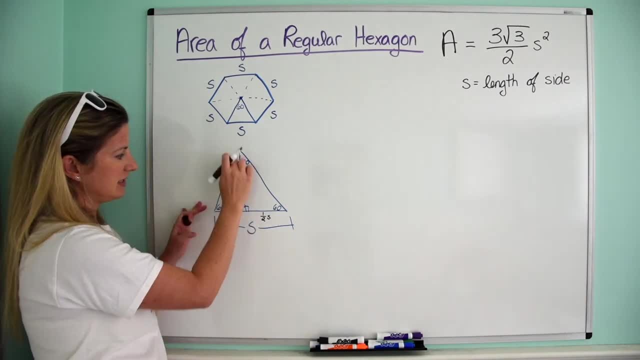 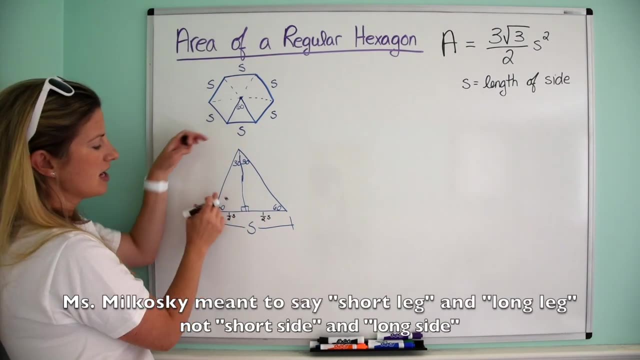 you bother breaking it up. Well, because I've created a 30,, 60,, 90 right here, with this being the short side. okay, This is the long side, This is the hypotenuse. Okay, So if I can get the long side, the measure of the long side, I now know the height. 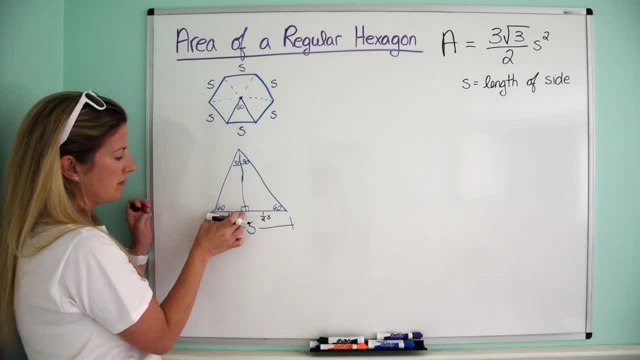 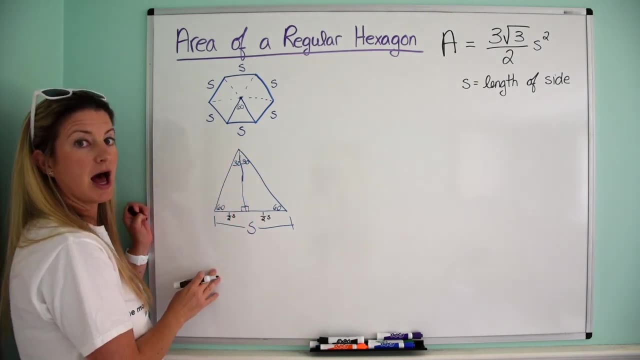 of this triangle? okay. So for 30,, 60,, 90s, if I am going from the short leg to the long leg, what do I do? I multiply by root three, okay. So if you click on a video right over there, 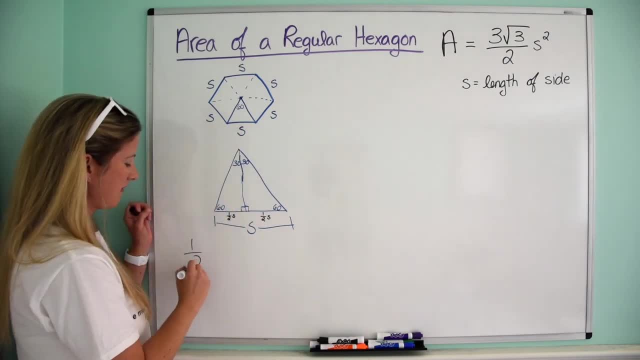 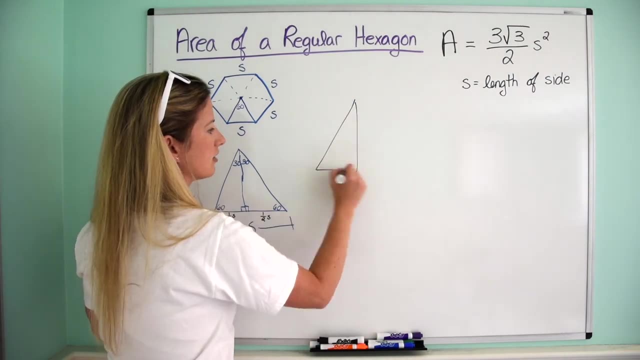 you can kind of see how to do that, okay. So I'm going to take my one half S, okay, because that's a short side. okay, And I'm going to multiply by root three, okay, Because, remember, in a 30,, 60,, 90,. so this is 60,, this is 30 here, this is 90,. okay, This is. 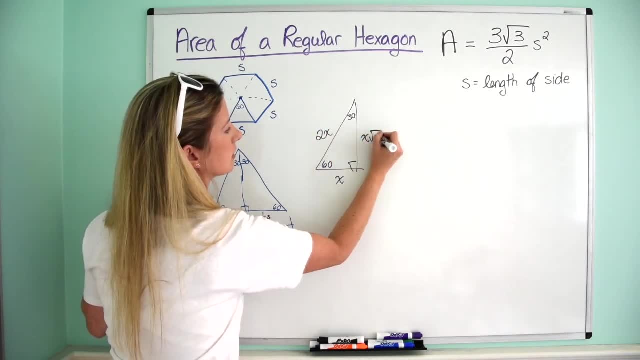 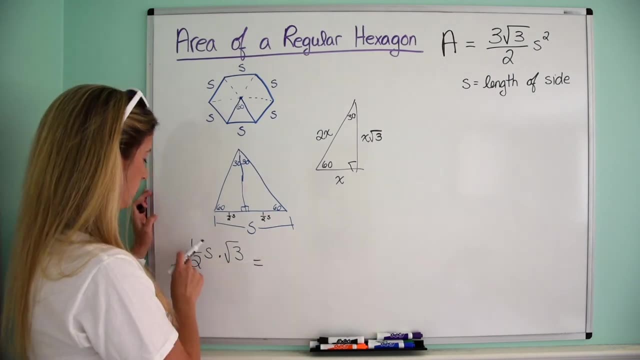 X, the hypotenuse is 2X and this is X root three. okay, So whatever this is, I multiply it by root three to get the long side. So I take one half S and I multiply it by root three, which is going: 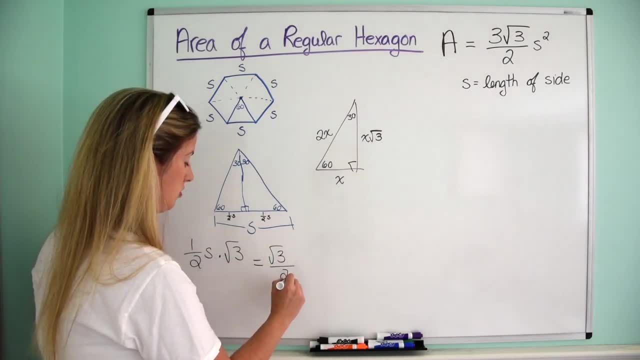 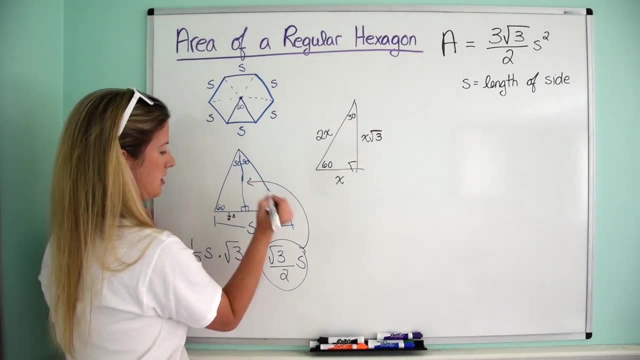 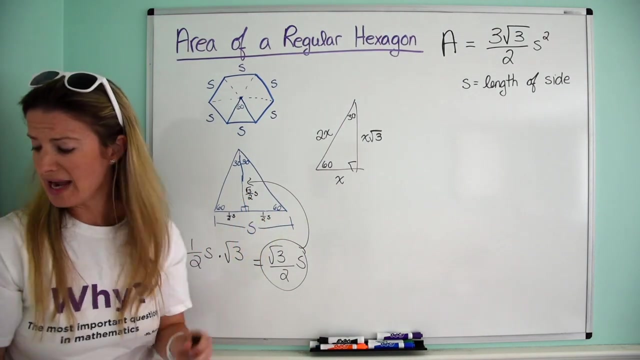 to just equal root three over two S, okay. So that's going to be my height. This right here is my height, okay, So I can write it right here. So I can write it where we got root three over two S, okay. So now I know it's super-duper messy. 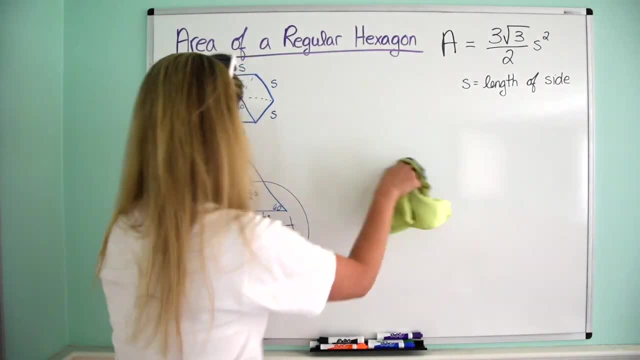 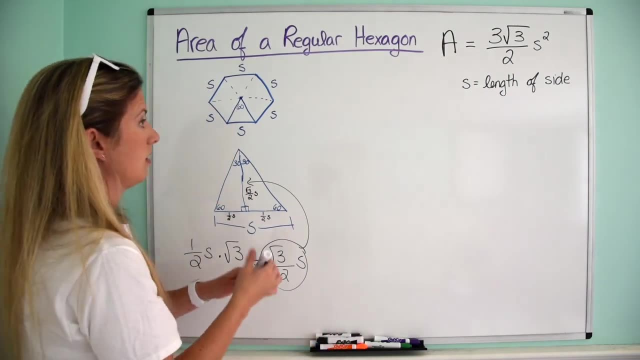 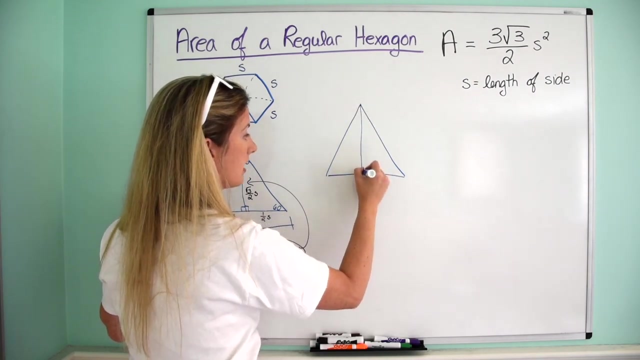 what I've got going on here, So let's clean it up, maybe again. So now I'm just going to redraw this triangle, okay, in blue, okay, over here. okay, So I'm going to redraw the big blue triangle that I had because, remember, my goal is to find the area of this, okay, And I know that this is 30,. 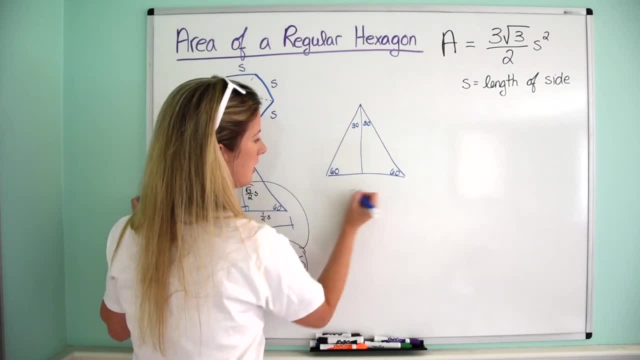 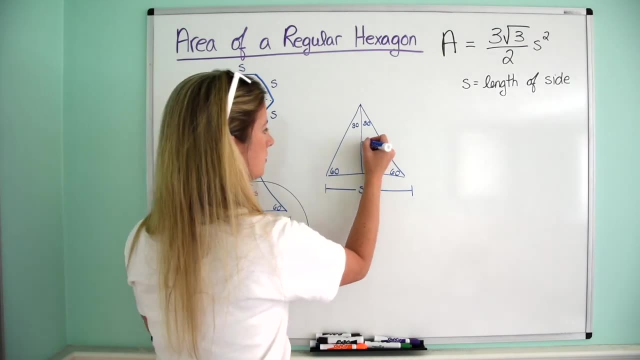 this is 30.. This is 60,. this is 60,. okay, This whole. the base of it was S and I know that the height is root three over two S, okay, So if I want the area of this triangle, I just know that it's one. 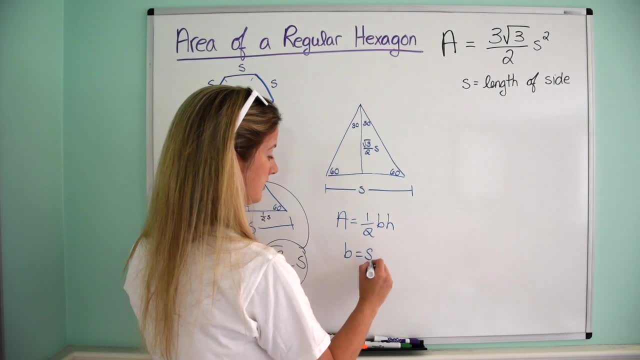 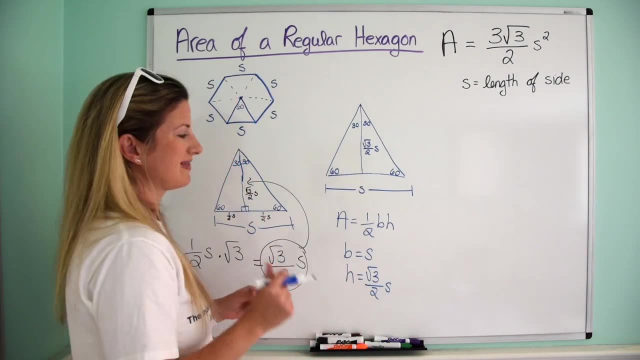 half base times height, And in this case the base is S and the height is root three over two S. okay, So if I want the area, all right, I'm just going to say: well, then, the area is. 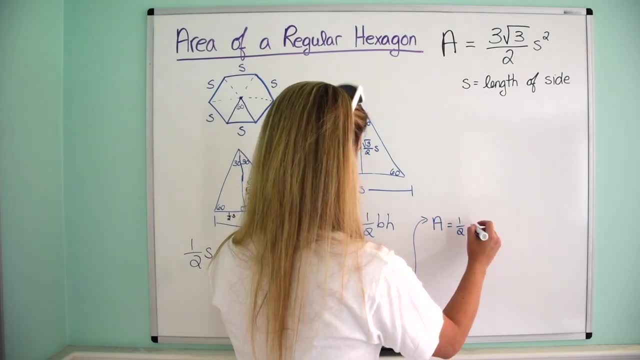 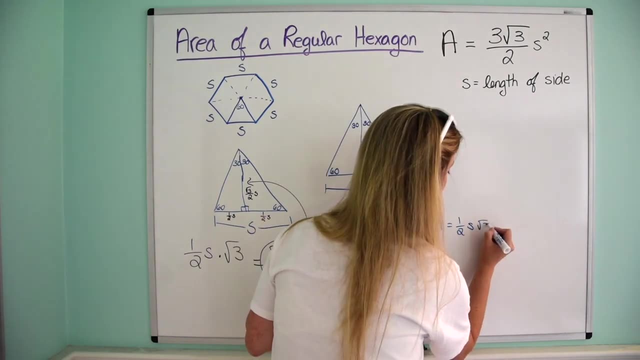 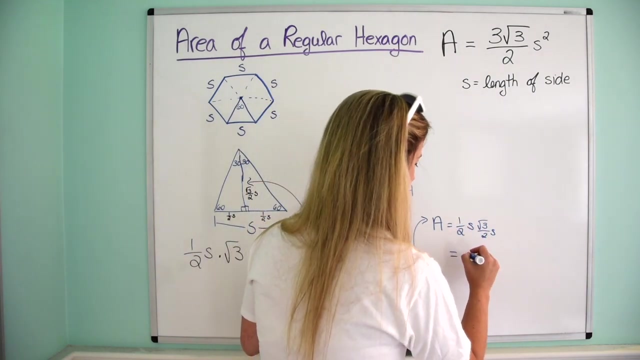 if I kind of come up here. so the area is just one half base, which is S okay. times height, which is root three over two S okay. So then I multiply all that together, I've got one times root three, which is just root three. two times two is four, and then I've got S times S. 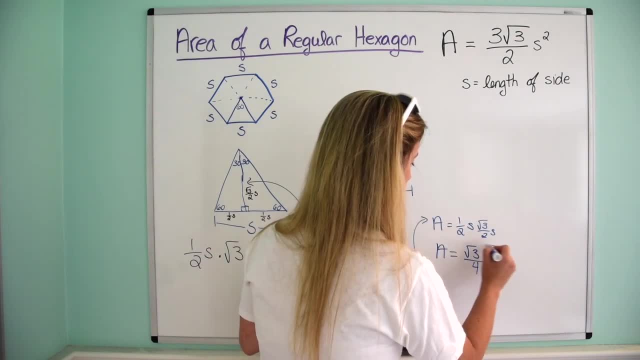 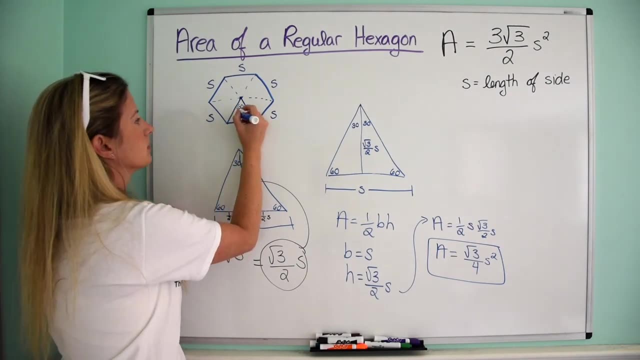 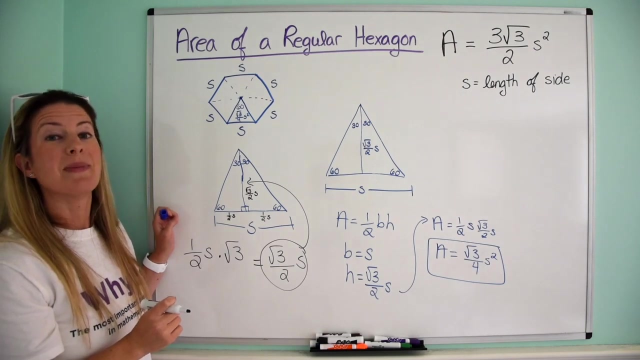 which is S squared. Perfect. So the area of this triangle? okay, right here, this triangle is root three over four S squared. So I'm just going to write: root three over four S squared is going to be the area of that. Well, how many do I have? How many of these triangles do I have? 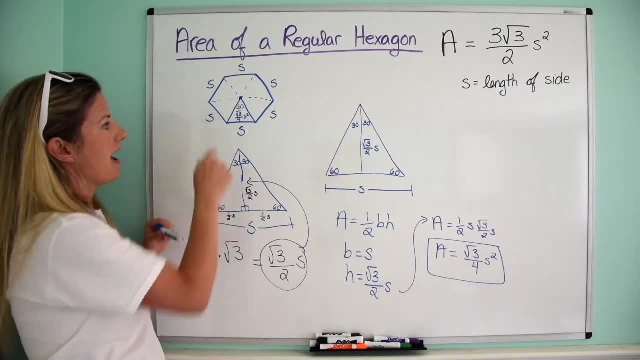 Remember, they're all identical because I've got a regular hexagon here. I have one, two, three, four, five, six, okay. So all I'm going to do is say, well, if one of them has an area of root. 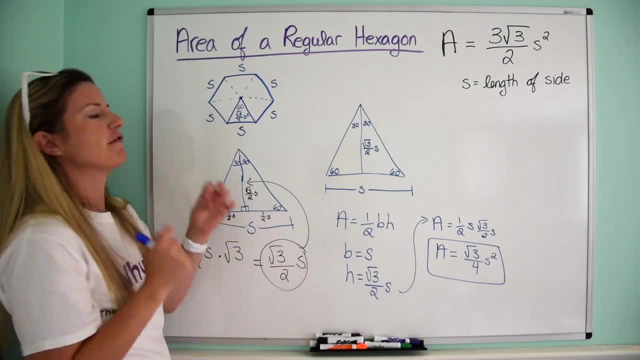 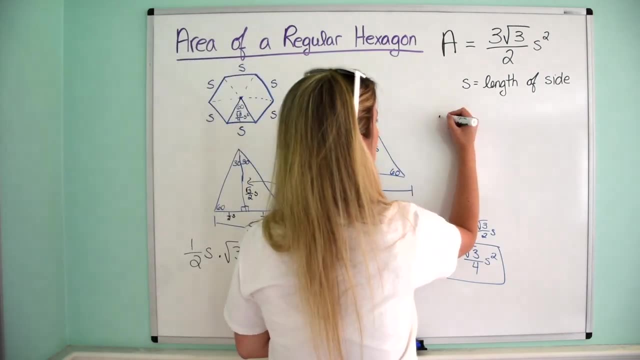 three over four S squared, then six of them have an area of root: three over four S squared times six. okay, So let's take another and we'll say: we'll come over here and we'll say the whole hexagon. 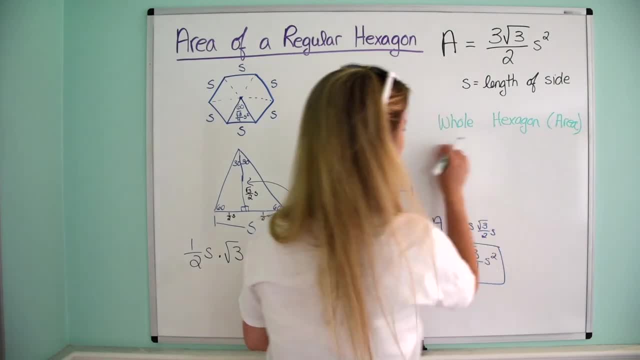 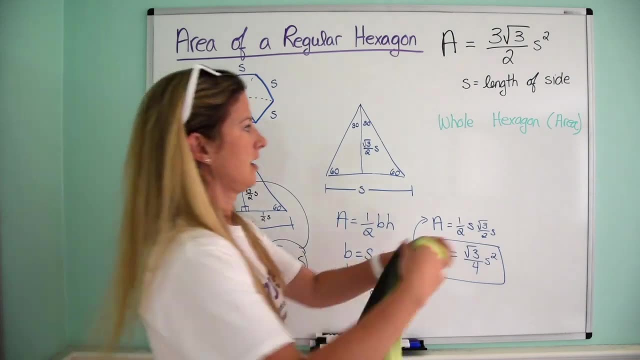 And then I'll just say area. I probably should have said area of the whole hexagon, but I think you know what I'm talking about here. Yeah, maybe I'll just write that, okay. So area of the whole hexagon, just in case you know. for those of you that are skipping around, 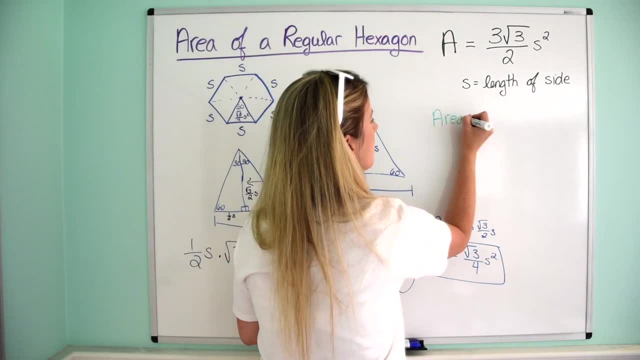 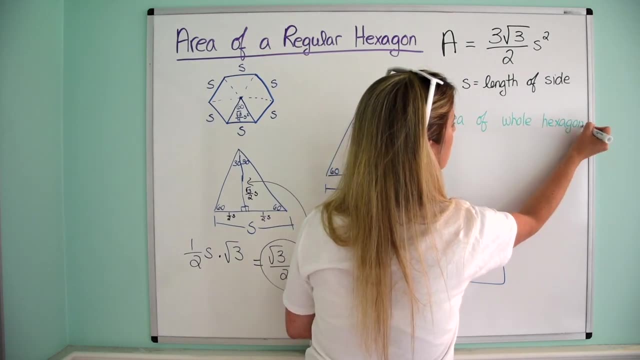 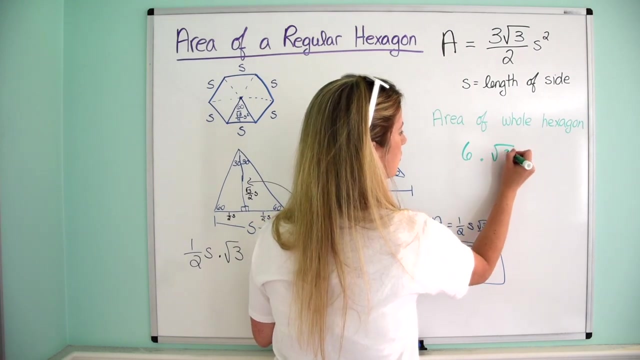 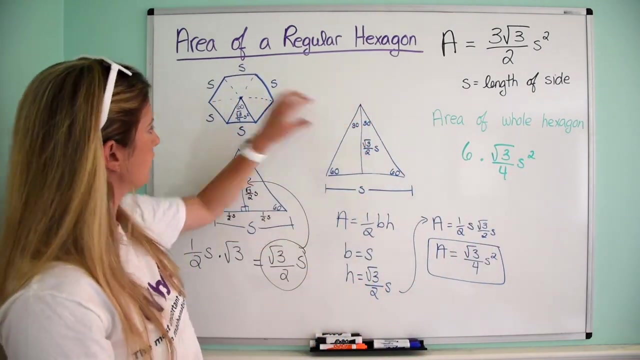 in the video and aren't watching it all the way through. So, area of the whole hexagon, Perfect, okay. So what I'm going to say is it's going to be six times root, three over four S squared. okay, So, because remember the area of one of them. 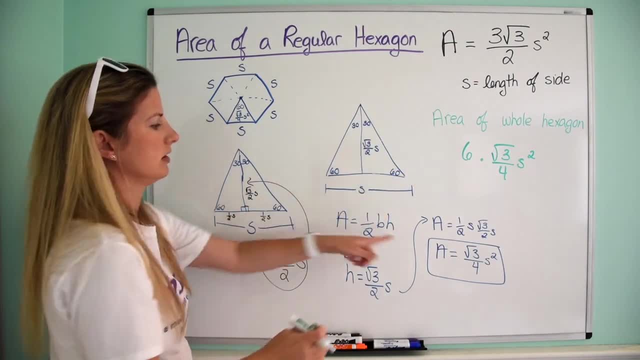 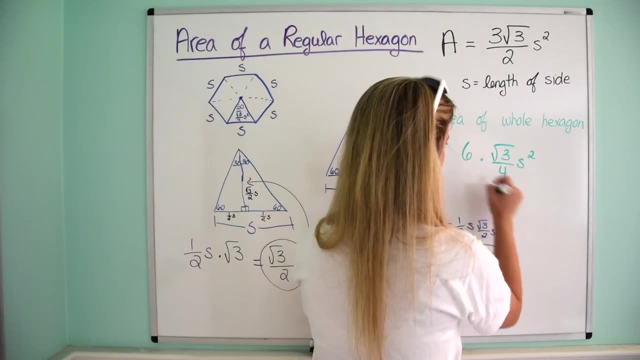 this triangle we pulled out and put over here and we said the area of this triangle is root three over four S squared. So then I just multiply it by six. So then that's just going to be oops. I'll come kind of down over here where I have room. So it's going to be six: root three over four S. 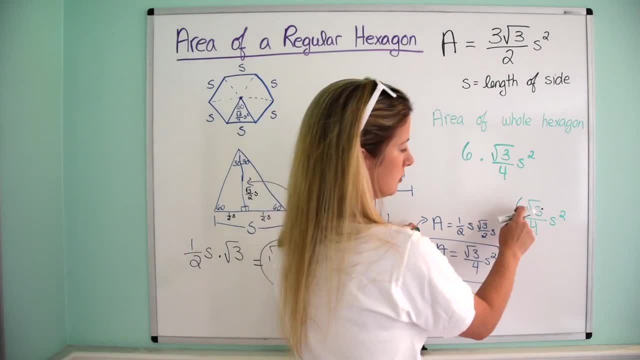 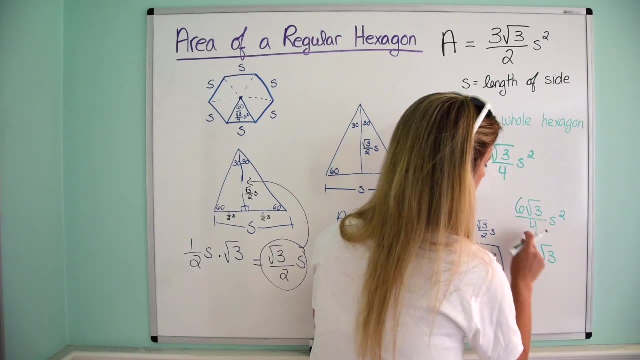 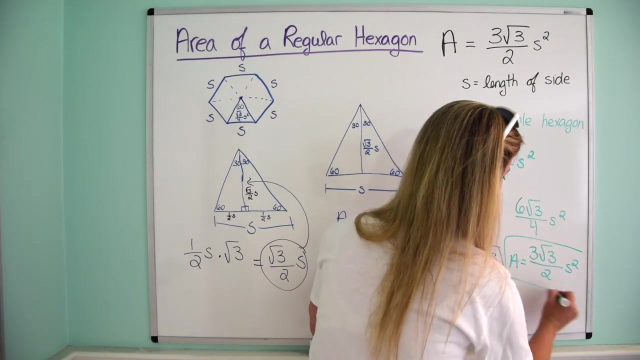 squared, And then obviously both six and four are divisible by two. So six divided by two is going to be. we can get rid of a two here. So that'll be what: Three root three, four divided by two is two S squared. Perfect, I'll write it as A equals, okay. So now we cross our fingers and 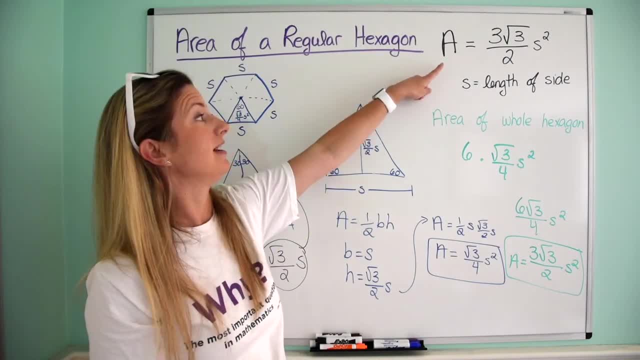 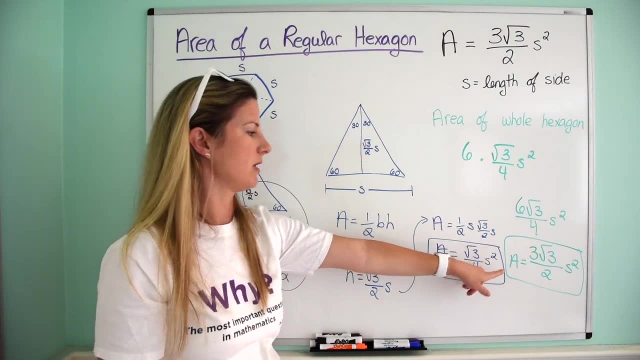 say: did we do it right? We did all this work and we did Look at that, Yep, So we knew this was a formula. I told you this was the formula to begin with, but I said: let's derive it, Let's see where it's coming from, okay, And there we have it. So the area: 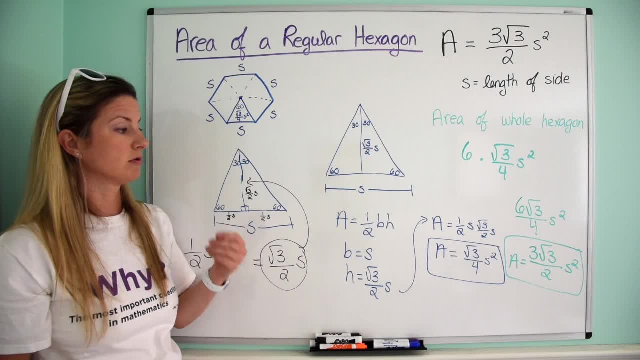 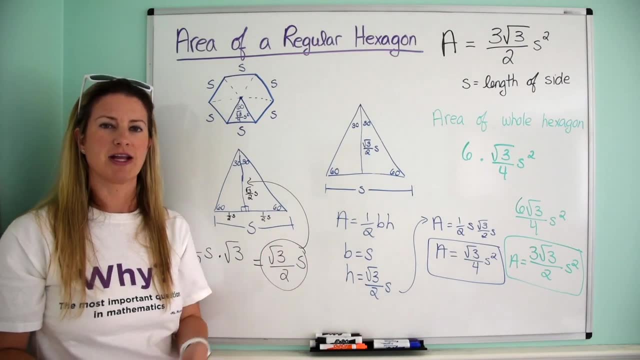 of a regular hexagon is going to just be three root three over two times S squared, the side length squared. And if you go to that problem that I have, where it's find the area of the regular hexagon with side length seven, you can actually just plug in seven for S squared. 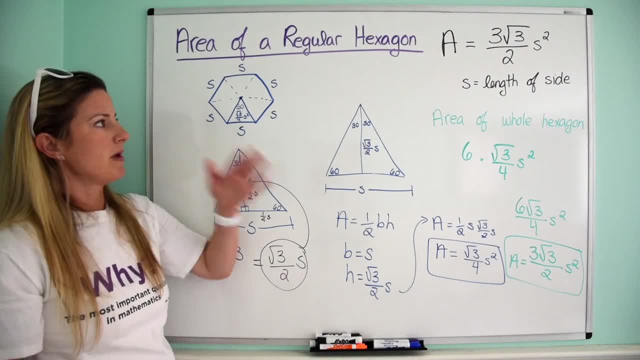 and you'll get the same answer that I get in the video. Now, remember, this is kind of a shortcut. You could also use it to find the area of the regular hexagon, but I'm going to use it to find the to check and stuff like that. But it is super duper important that you understand where it. 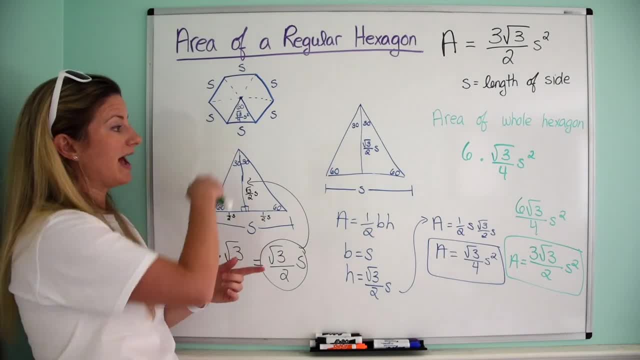 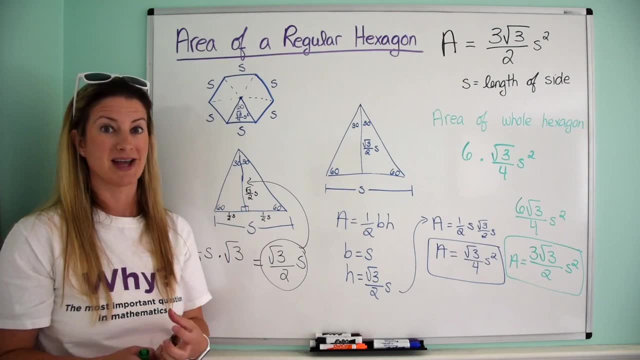 comes from, And you do have to be prepared that sometimes your teacher will ask you to get the area of a hexagon the long way. Even I did that in class because I thought it was important for kids to understand where it's coming from. okay, So you can almost use this as a check, maybe after.